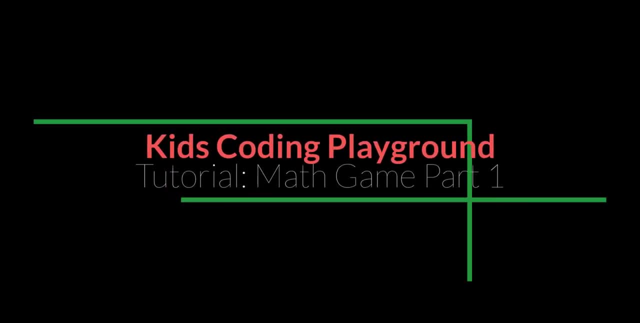 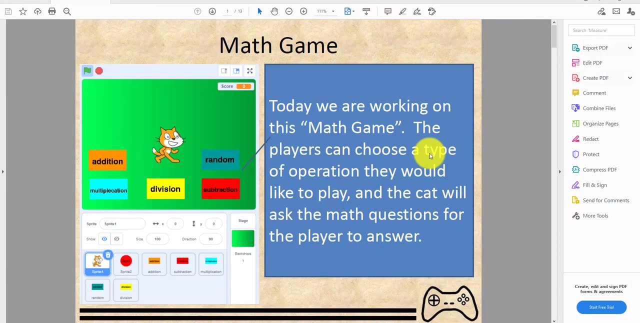 So welcome back, guys, to another tutorial on Kids Coding Playground. Today we'll be doing a math game So the players can choose any operation, such as addition, multiplication, division and subtraction, Or you can pick a random operation, So we'll choose a random one for you to play And the player can choose a type of operation and they would like to play And the cat will ask the math problem. 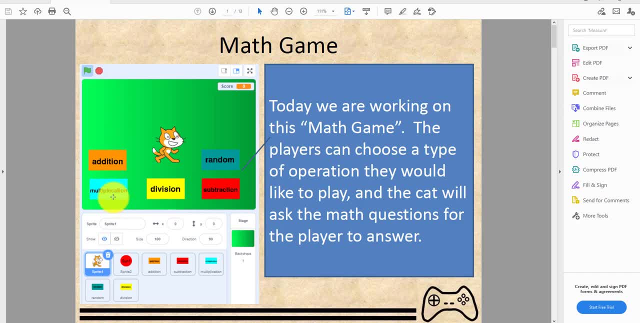 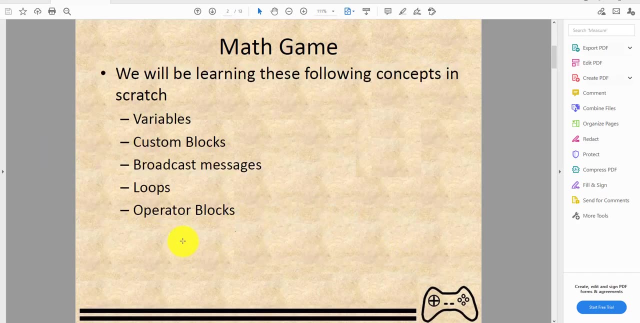 For each operation. So let's say, you click on multiplication, The cat will start asking questions for multiplication. If you click on subtraction, the cat will start asking questions for subtraction. So today we'll be learning these following concepts in Scratch: Variables, custom blocks, broadcasting messages, loops, and we'll be using a bunch of operator blocks. We can later expand this math game into a math racing game, which I did for my 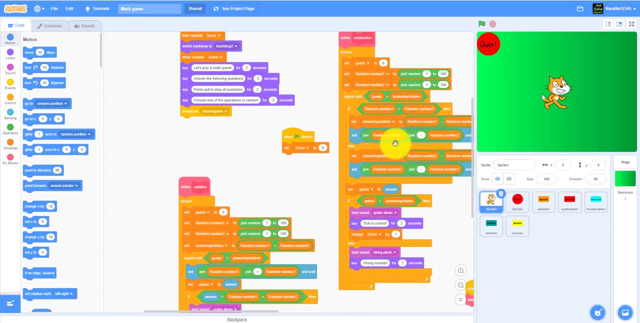 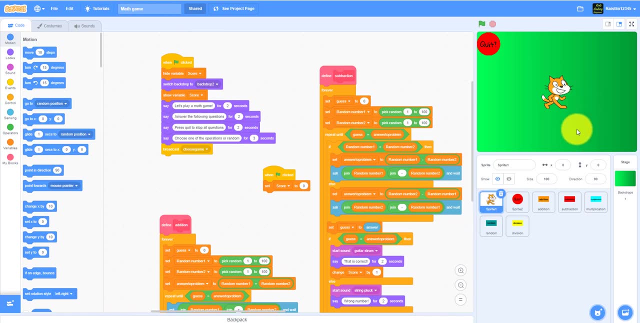 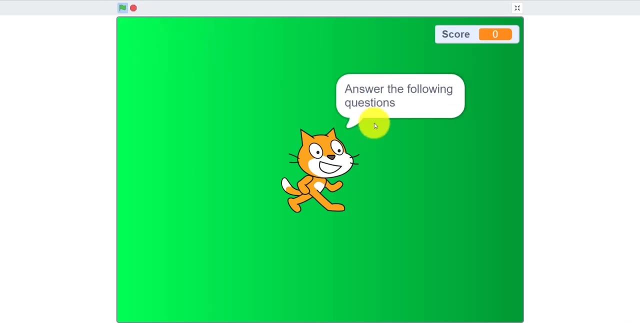 tech fair about like two years ago and I got third place on the tech fair. So later we can expand to that. But first we'll need to work on the regular math racing game, math game. So I'll demo the game for you guys. So in the beginning I'll just say: let's play a math game. answer the following questions. press quit to stop all questions. That's just a stop all. choose one of the operations or random. So let me show you: when you click on random, it'll pick a random operation for you, As you can see. 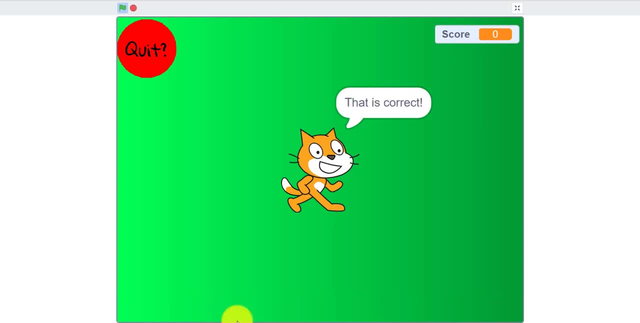 So I'm just going to. so when you get a question correct, you'll say: that is correct. And let's say, if I get a question wrong on purpose like, you'll say wrong number And there's also different modes. Today we'll be working on addition and subtraction. I think that's all we'll have time for. We'll work on multiplication and division in the later videos. So let's see addition. So 33 plus 20, that's 53.. 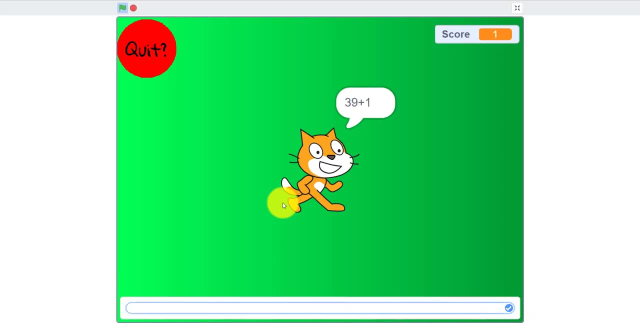 That's 40. So if you get it right, you'll get more score. As you can see in the top right corner, you can get more score. So, yeah, that's pretty much the game. So let's start a new project. 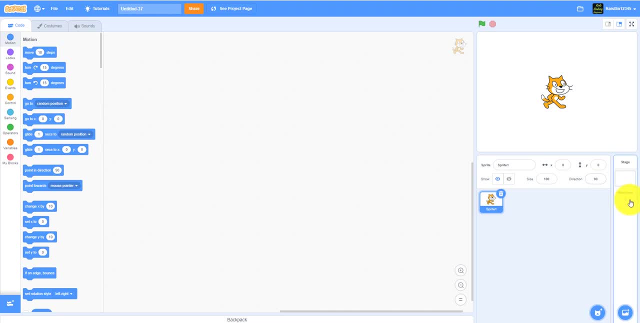 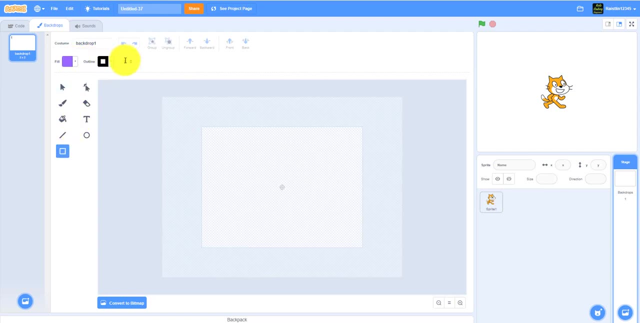 Okay, so we can keep the cat for now, And if you want to make a backdrop, you can. So I just made like a little green backdrop with no outline And I just like use the darker green on this side, like that, And I just drew a square. you guys can do whatever you guys would like. I'm just gonna make a backdrop, so it's going to be my backdrop and we're going to keep the cat. So this is going be my backdrop And we're going to keep the cat. I can rename it to cat, actually, But in the old one I just still had a sprite on. but um, and then we'll need to make some buttons. I already have them in my backpack. today we'll be making an article with cute, stronger women and more. 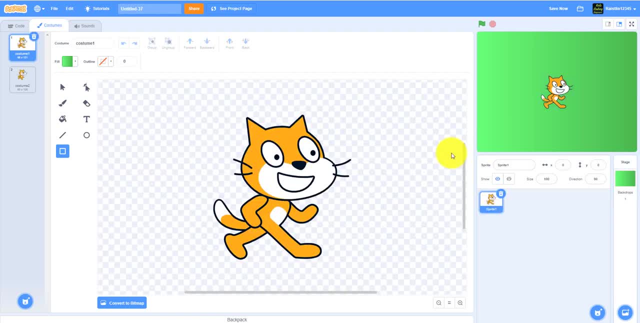 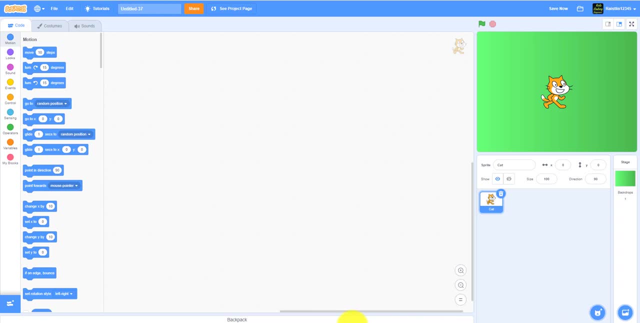 So this is going to be my backdrop And we're going here for some further details on this next project. We'll keep the cat. I just told you guys that I have my and we're have them in my backpack Today. we'll be making the addition and subtraction ones. 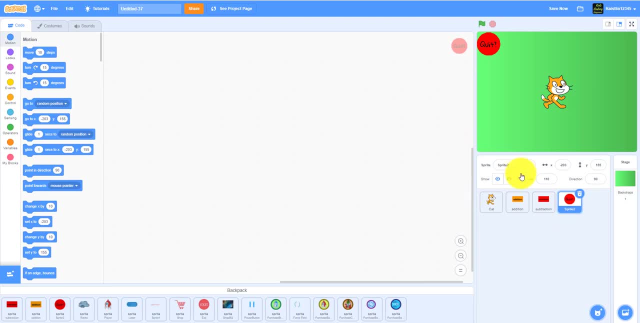 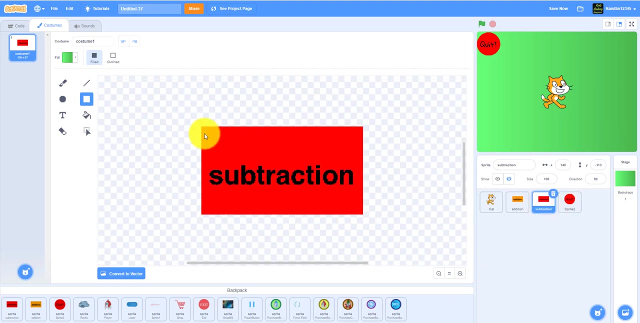 and the quit button. That's all we'll have time for, I think. So for the addition, all we did was just drew a square, a rectangle, and then wrote addition, and same for subtraction. we just drew a rectangle and then wrote the word subtraction, and then for the quit button, just a. 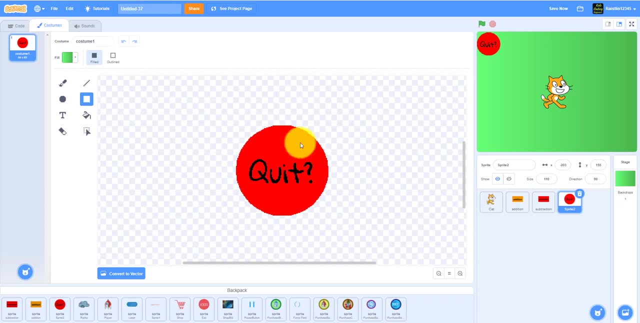 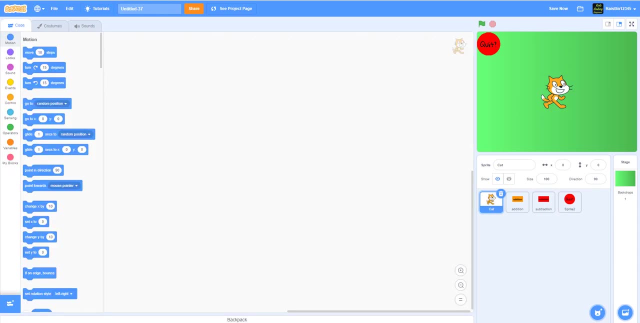 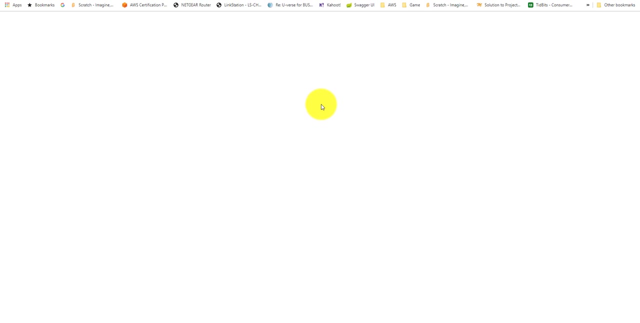 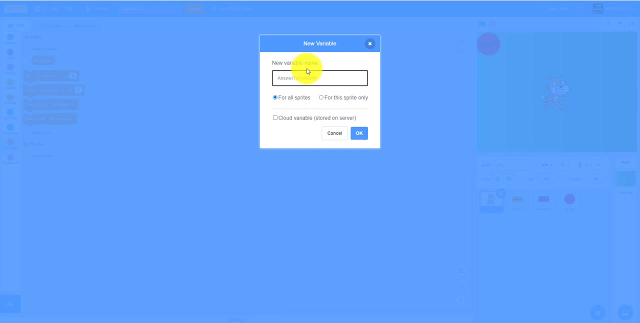 circle and then wrote quit. So that's it for the three buttons, and let's go work on the code now. First we need to create some variables, so we're gonna make a variable called answerToProblem. so make this answer, Como. your problem is for all sprites. 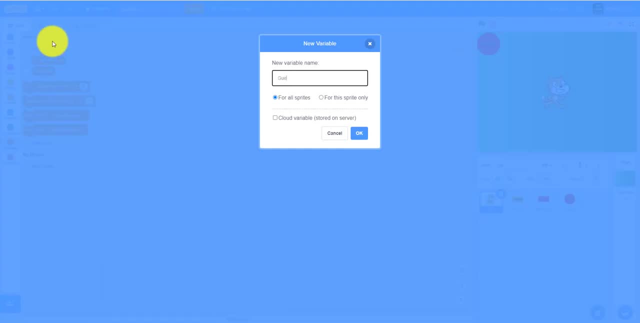 and then we'll need to make a variable, make another variable called guess, so this is what the player guesses as the answer. and then we have the random number one, which is the number picking, the random number, which is the first number they'll pick. and then we also have a second number, random number two, and then we'll need to 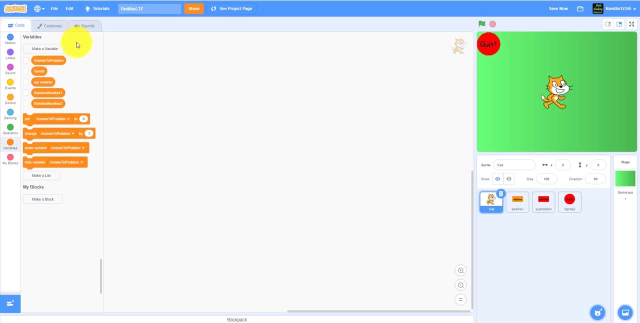 create one more called random game and score. let me create two more actually so random game. so this is for the um. so let's say you click the random button, it'll pick a random game, so this is what it's for- and then you have to make score and then we can delete my variable. this is not use. 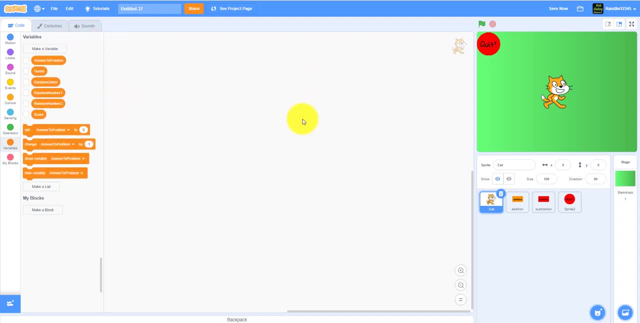 so this is all we have for now. so let's go to the cat, get a. one fly clicked. so one fly clicked. we're going to hide some variables. so, um, we're going to hide the variable score in the beginning. actually, no, we don't need this. we don't need to hide the variable, we can just keep it showing. i 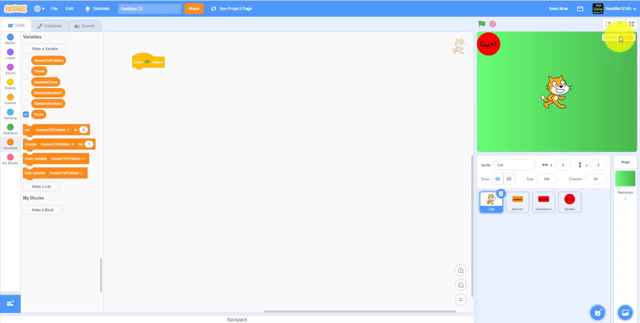 guess, if you want, i'm gonna keep the score on the right side, so i'm gonna get a one fly clicked and then i'm gonna um show the variable score. actually, no, we don't need that because it's already shown- and i'm just gonna make it. say, let's play a math game. 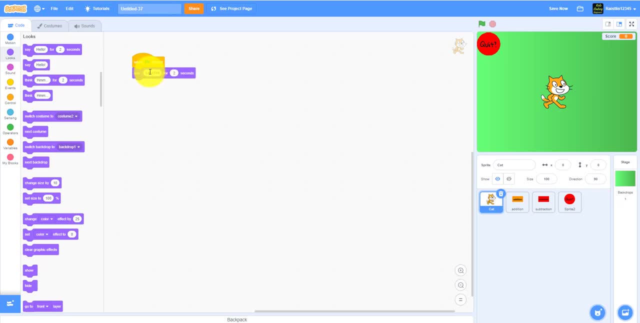 math game. so let's play a math game. i'll say it for like two seconds and then i'll duplicate it. we're just gonna tell them the instructions how to play in the beginning and then i'm gonna say: answer the following questions. and then i'm gonna do it duplicate two more. one is: press quit the quit button. 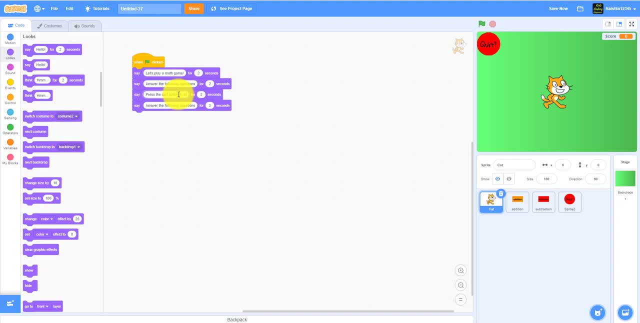 to stop all question, stop all questions. so this is just a stop all, and then one more we'll do, choose one of the operations or random. so this: these will be the instructions. so if you guys want to make it um less, less, like less saying, then you can just put all the instructions and 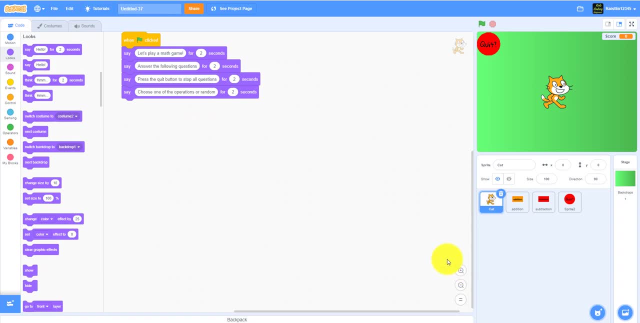 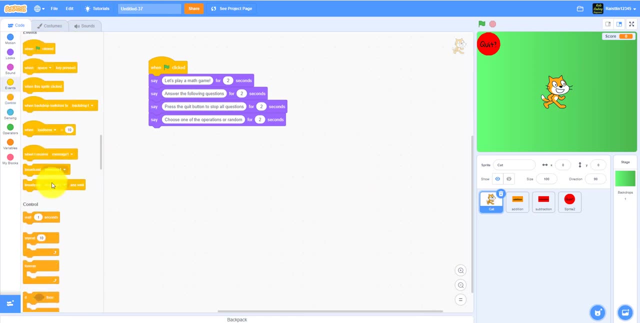 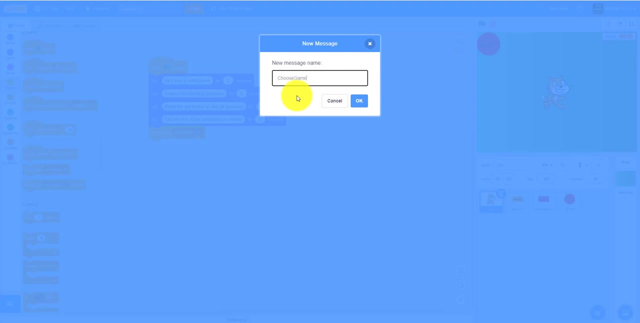 Wednesday and just make it for a longer time. so I just did it like this, but you guys can do it any differently, so I'm gonna make a new variable right now. I mean new broadcast. I'm gonna name it shoes game. so this is just to uh select. 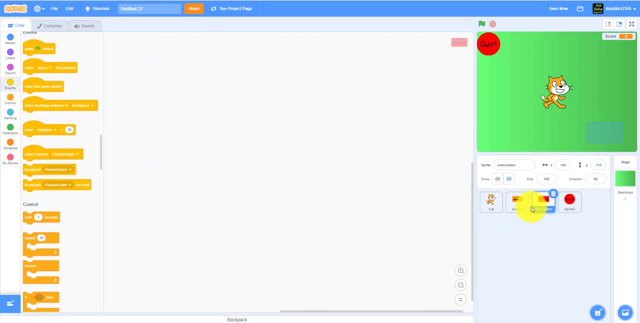 the game. so choosing game. so let's go into our addition and subtraction. so for addition, I'm gonna get a winner receive choose game we want to show, so it'll show up in the beginning. and in the beginning we want to hide one flag. click you want to hide, sorry, hide. so I'm gonna zoom in a little bit when I when 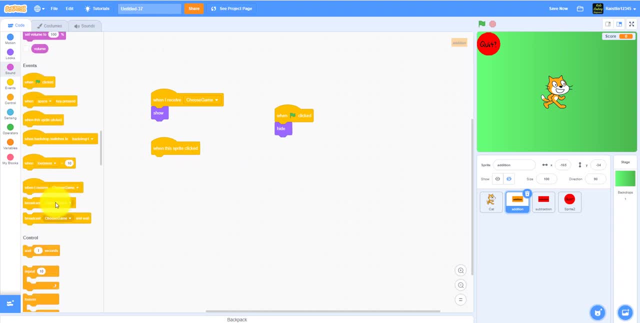 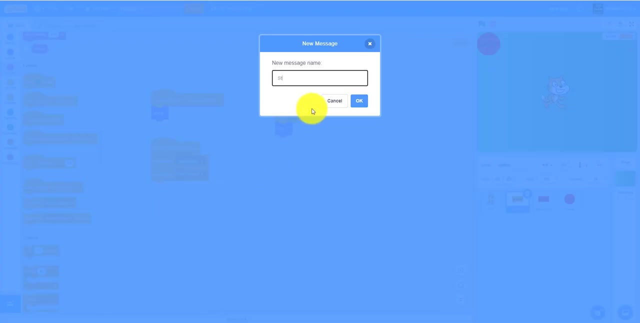 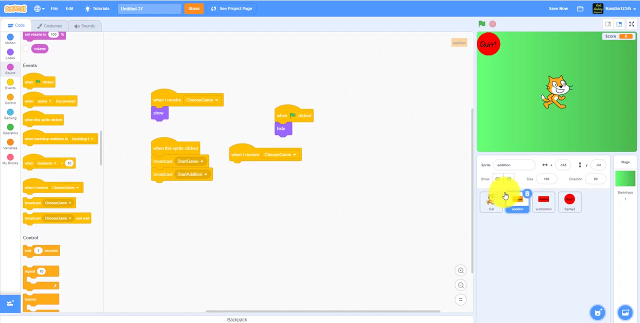 this sprite is clicked, so I'm gonna do two more broadcasts. one is called start game and one is called start addition, and we'll make another one called start addition, letting the player know it'll start the addition, start addition. and then, when I receive start game, we want to hide the button. is. 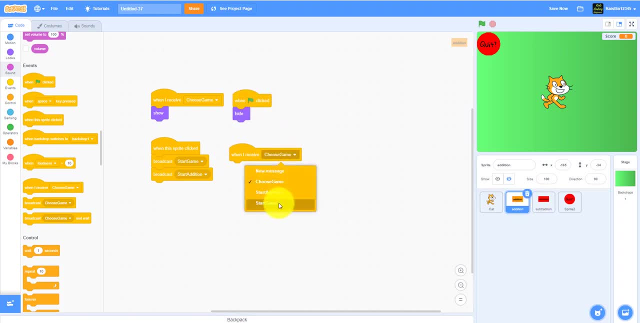 no longer needed after the game has started. start game: we want to hide and then, um, this part is not necessary, but you guys can add it if you would like. it's just to make your game look better, so when you put your mouse on it, it'll. 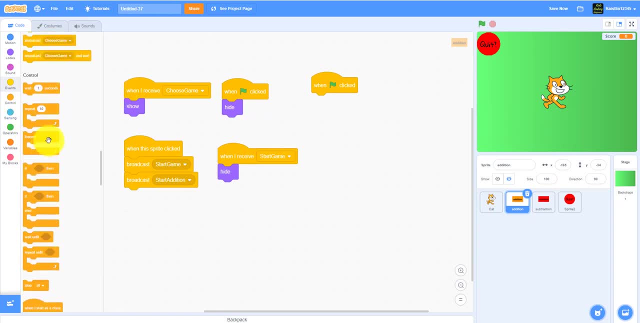 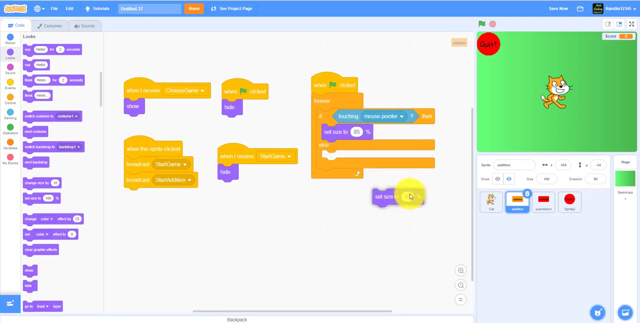 get bigger and smaller, so just get a forever loop. if touching mouse pointer, then we can set the size to 85%, we can set the size to 85%, Else set it to 100. there are many other ways to do it, but the other ways are a. 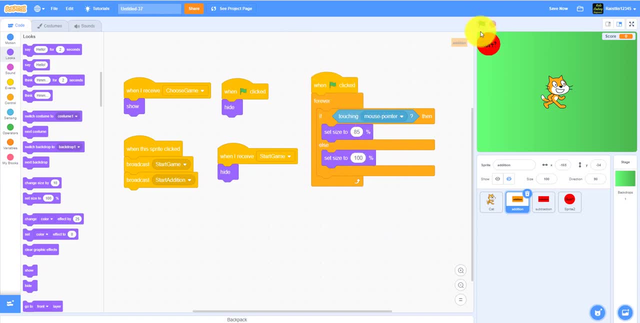 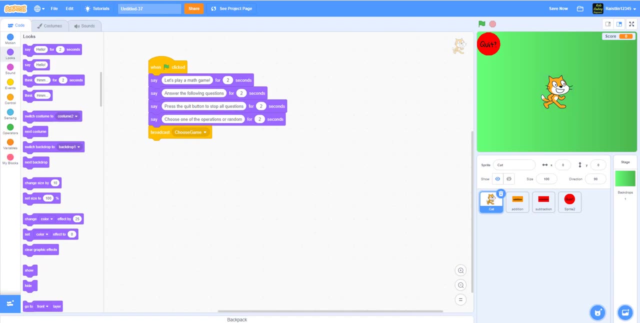 little bit more difficult. so this is just an easier way of doing it. so now let's go back to the cat. so for the cat we're gonna have to make some custom blocks. so this is just an easier way of doing it. so now let's go back to the cat. so for the cat we're gonna have to make some custom blocks. 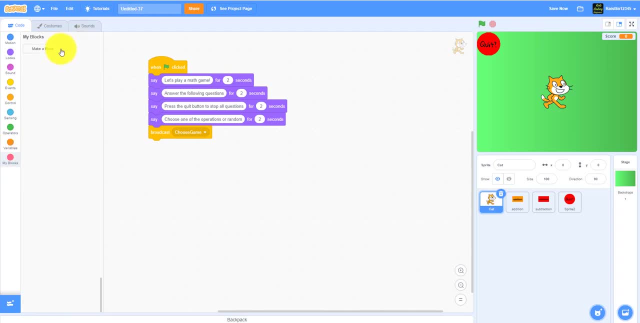 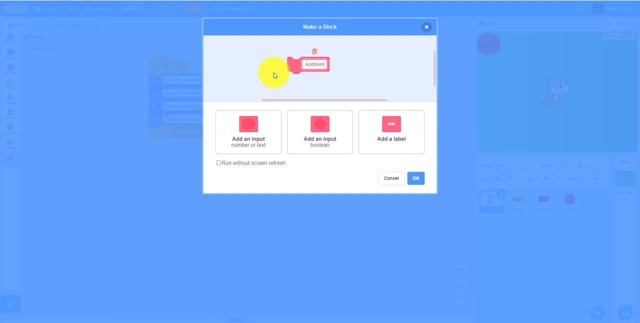 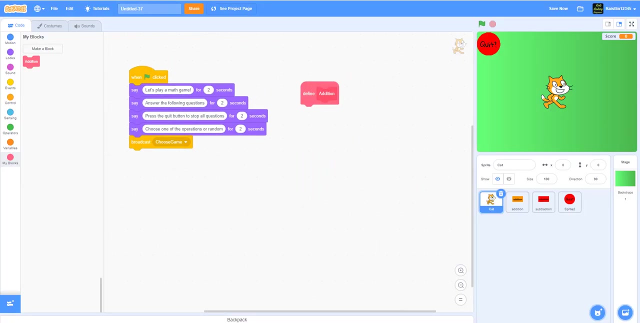 So we're going to get a new custom block. let's name it addition. so we're going to define the addition block. So let's define the addition block right now. let's get a forever loop And then in the beginning we want to set the guess to zero. 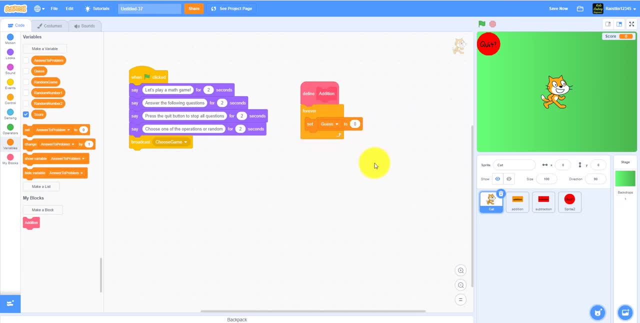 So the guess is zero in the beginning, So we set it zero. And then we want to set the random number one to pick: random one to 100. So, for addition, it will pick random one to 100. So pick random one to 100. 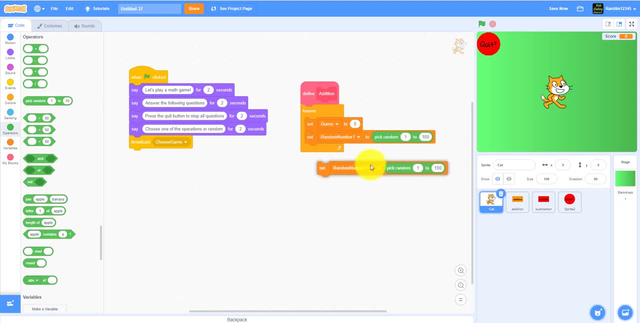 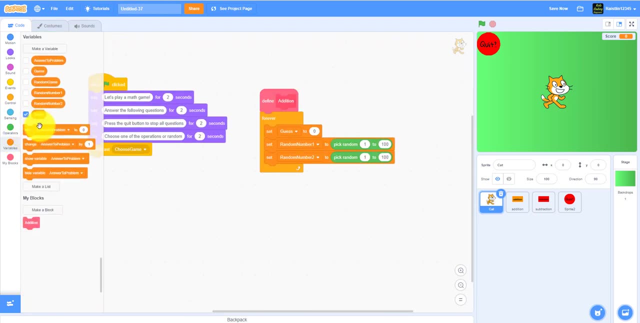 So the first number will pick random one to 100. And then we want to set the second number- pick random number two- to also pick random one to 100. And then we're going to use the variable set answer to problem To random number one plus the random number two, which is the first number which you. 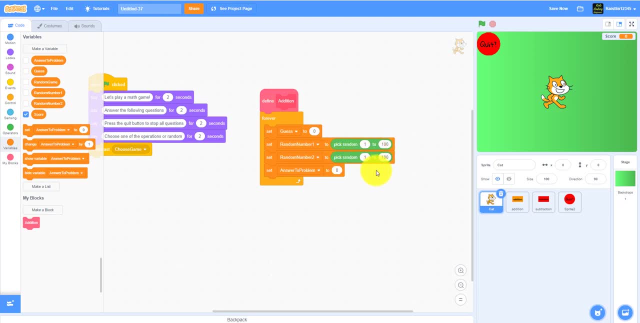 pick random. it can be like 25 or something, And then the second one can be like 10.. And you add them together So you get an addition operator. So you add the random number one which is a random number. pick one to 100.. 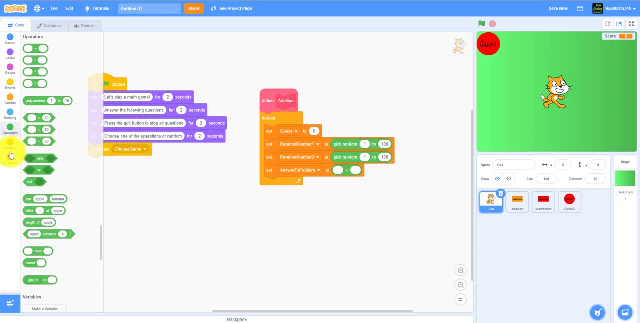 And random number two, which is a pick, random one to 100.. So you add them up. oops, put that back in like random number one plus random number two, And then I'm going to zoom in a little bit more so you guys can see it better. 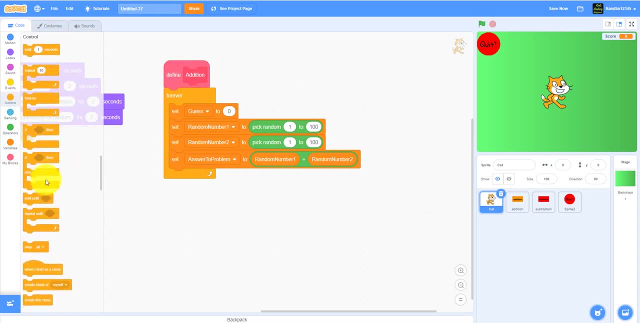 And then we're going to get a repeat until So we're going to repeat until guess is equal to answer to problem. So it will repeat until the answer is right. So the guess is what the player inputs And the answer to problem is the answer to the problem, the random number one plus the. 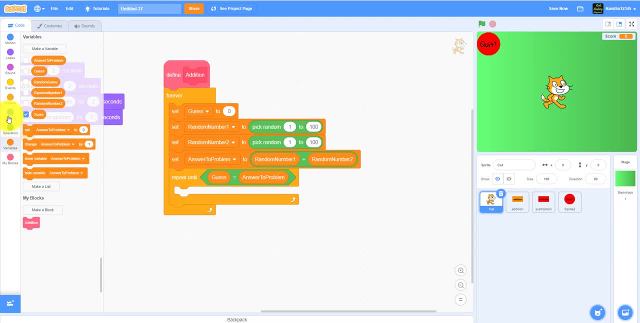 random number two. And then we're going to ask, Ask, Ask. join random number one. join the add addition symbol random number two. So it will ask: what is random number one plus random number two? So we're going to join, just pop that in there, get in another join. 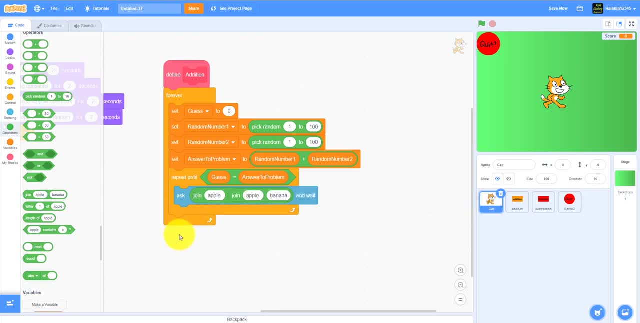 We need two joins and put it in here. So we're going to join the random number one Addition symbol And then random number two with that. So ask that, And then, and then after that, we want to set the guess to the answer, which is the. 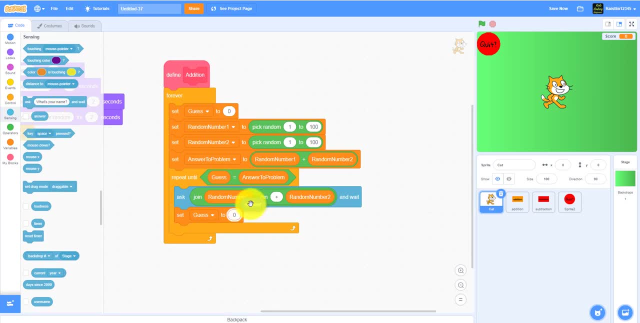 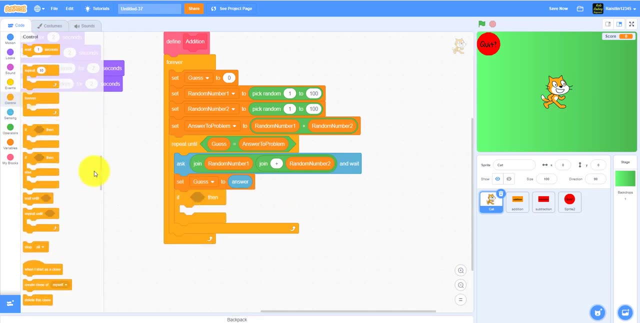 answer right here the correct answer, And then if the answer is equal to random number one plus random number two. So this is just to check if the player has got the right answer. So if random number one Is equal, If the answer is equal to random number one plus random number two, 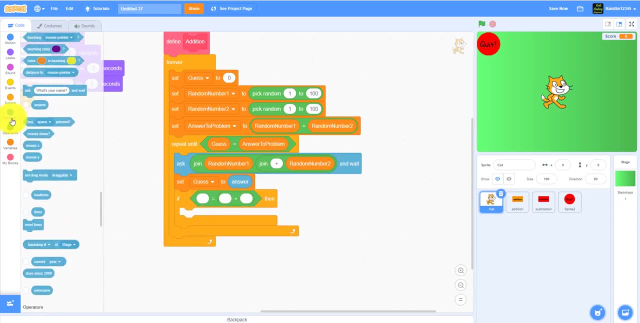 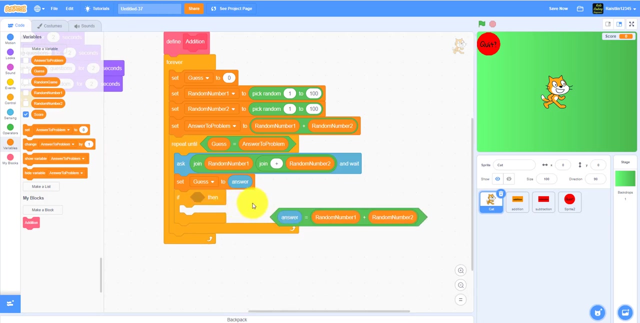 So we'll get an addition symbol. If the answer is equal to random number one plus random number two, then we can start. Actually, this should be an if-else statement, because if they get it wrong then it should say wrong number. 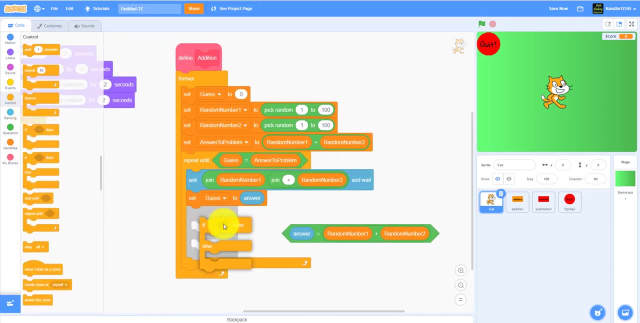 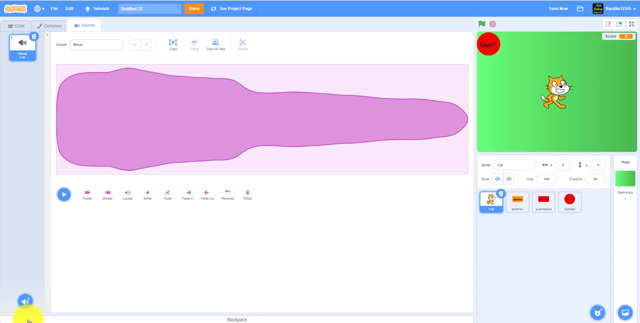 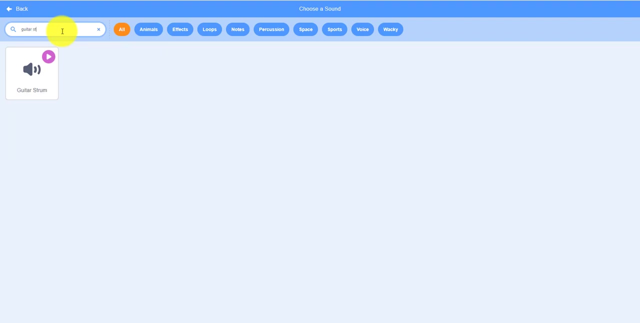 So let's change this to an if-else. Sorry about that. So you put that in here and then when I get something right, I'm going to get a new sound. So I got like a guitar strum sound, Guitar strum. 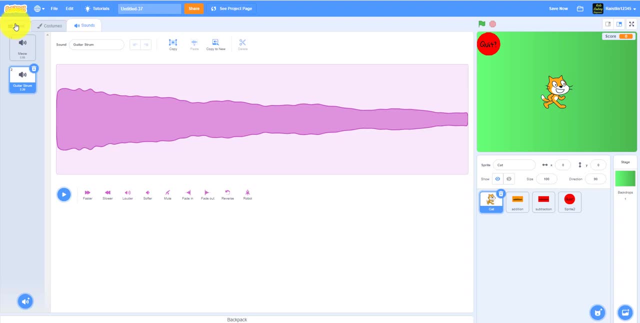 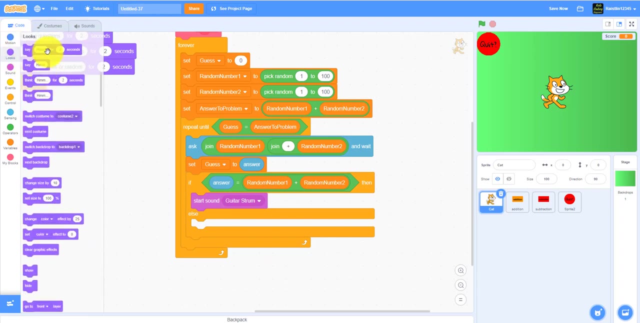 This one sounds like this, And then I just put in here: play sound guitar strum, and then it will say: that is correct, That is correct, That is correct for two seconds, And then we can change the score by one because they got the right answer. 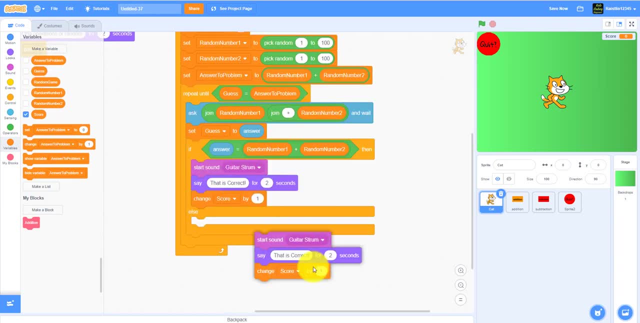 Else, if they get it wrong? oops, let me just duplicate this: If they get it wrong, then we'll say something else. We'll say: that is the wrong answer. And then, instead of playing guitar strum, I got like a string pluck sound. 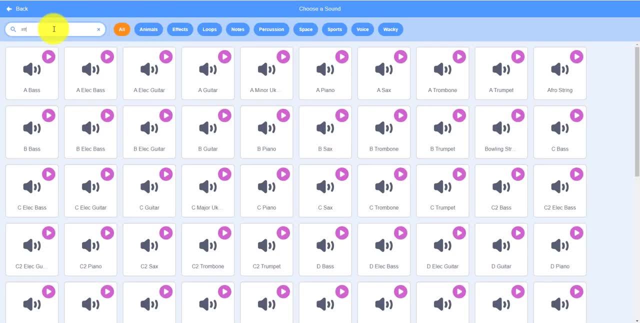 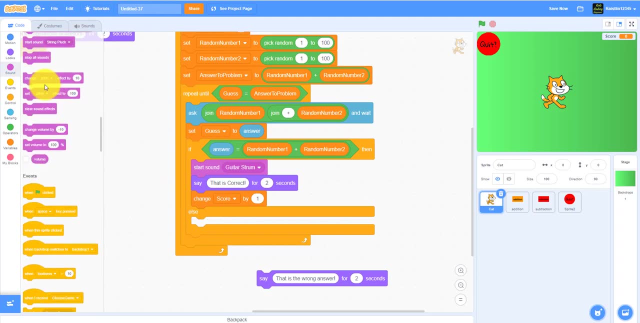 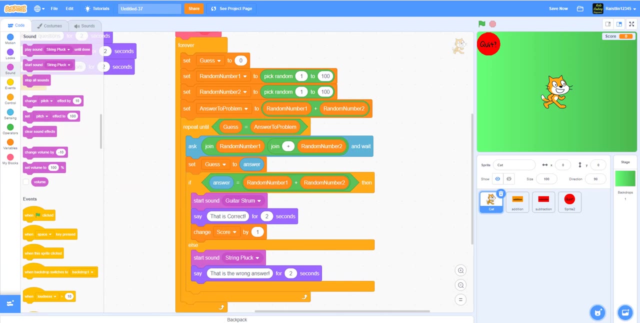 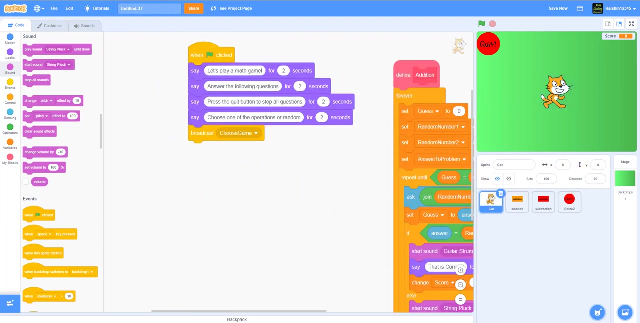 So I'm just going to go to sounds, put that right here and then say that is the wrong answer. Okay, And now we have to call the addition thing. So we broadcasted: start addition from here, Remember, right here. So I'm going to go to the cat. 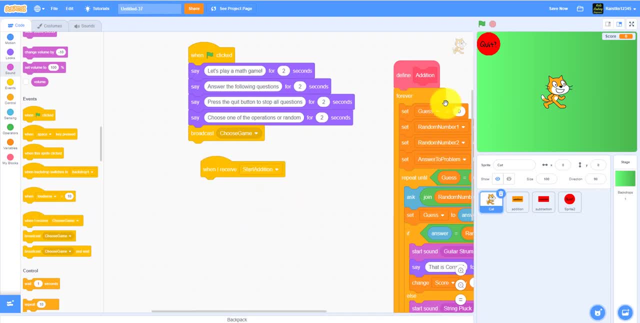 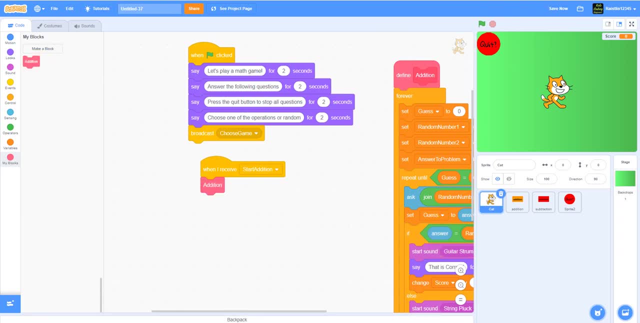 So addition. So now let's try out. Let's try it out. So it's going to say let's play a math game. Answer the following questions. Press the quit button to stop all answers. Choose one of the random operators. 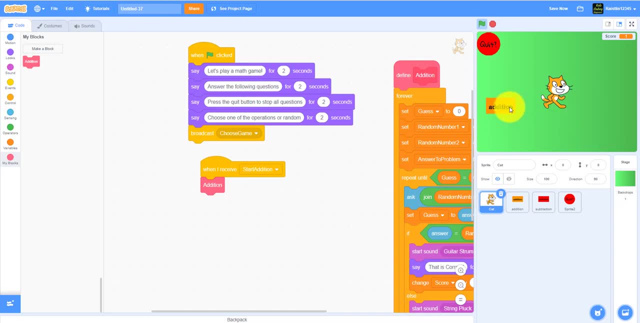 Operators are random, So we only have one operation right now. So let's click on addition, So ask the answer, as you can see right here. So 54 plus 42 is equal to 96.. So let's put 96..